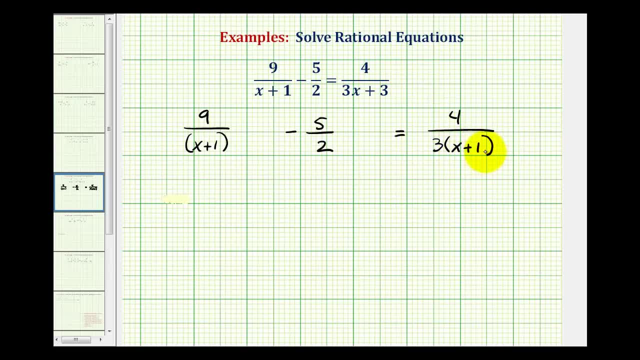 So we can write this as three times the quantity x plus one. Now, looking at the denominators, notice how the LCD would have to contain a factor of two, a factor of three and a factor of x plus one, So two times three times x plus one. 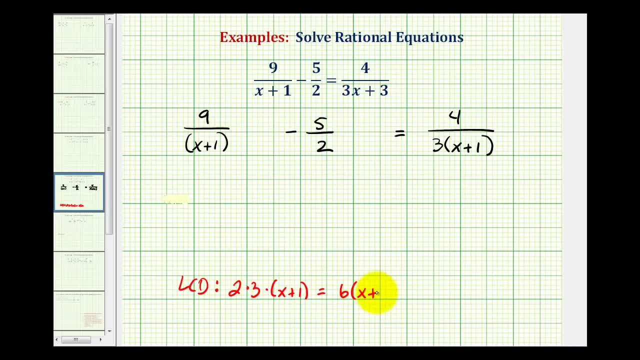 So the LCD would be six times the quantity x plus one. So now we're going to multiply each fraction by the LCD. We are not going to obtain a common denominator for each of these fractions, which is often a common error, So we'll multiply each fraction by six times the quantity x plus one. all over one. 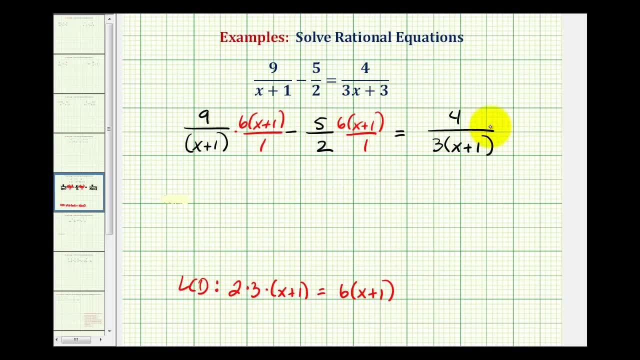 So six times the quantity x plus one, One over one, And times six times the quantity x plus one all over one. Remember, if we multiply both sides of the equation by the same thing, it does not change the solutions. So before we simplify and multiply and then solve this, we should take a moment to list the excluded values or the values that x can never be. 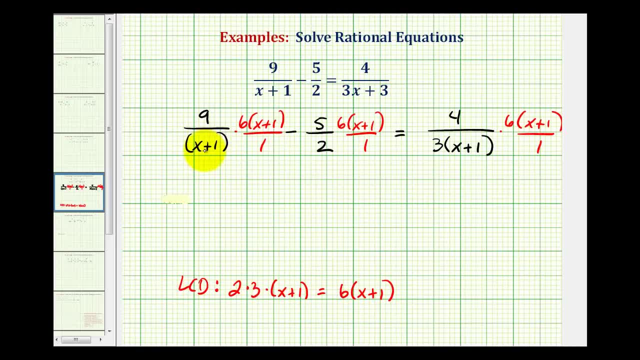 And since we can never divide by zero, we know x can never equal negative one, here or here. So our excluded value is: x cannot equal negative one. If, when solving this equation, we get a solution of x equals negative one, we must exclude it. 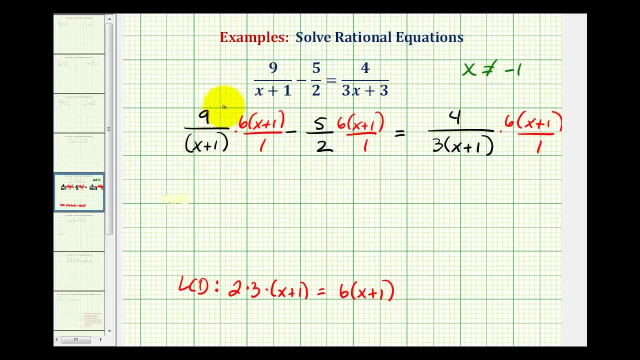 Now, before we find these products, let's simplify. Notice: for this first product, we have a factor of x plus one over a factor of x plus one, So now the denominator is equal to one and our numerator is nine times six, So now we have fifty-four minus here, a factor of two simplifies. 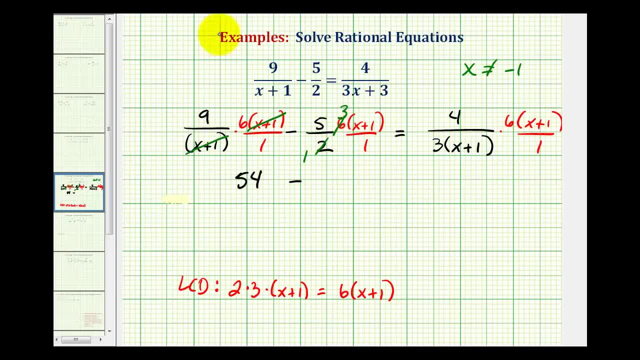 This simplifies to one. This simplifies to three, Leaving us with fifteen times the quantity x plus one equals. on the right side, we have x plus one over x plus one. That simplifies to one. Six and three share a common factor of three. 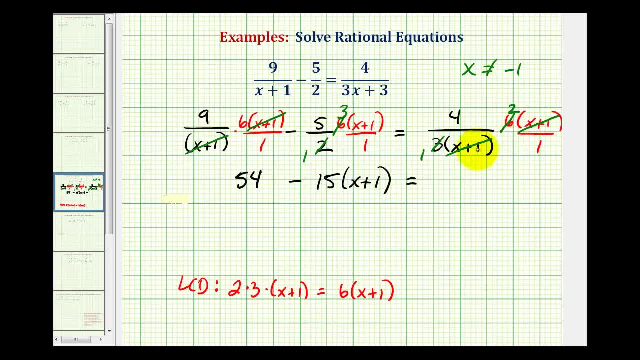 This simplifies to one. This simplifies to two. Again, notice: our denominator is equal to one, leaving us with just four times two, which is equal to eight. Notice the result of multiplying every fraction by the LCD eliminates all of the fractions and now we solve the resulting equation.